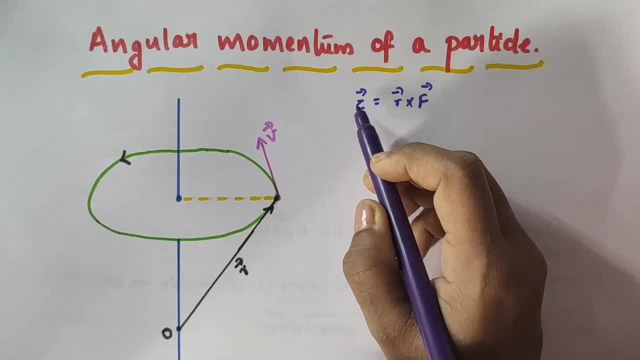 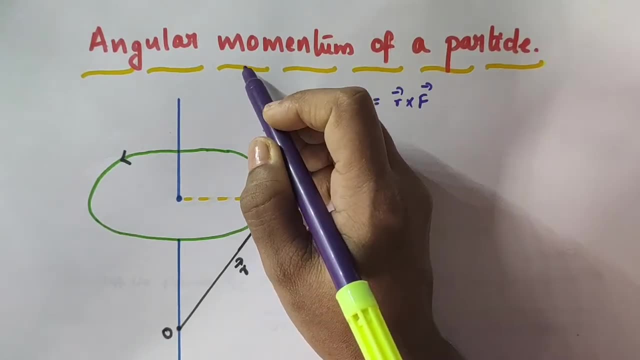 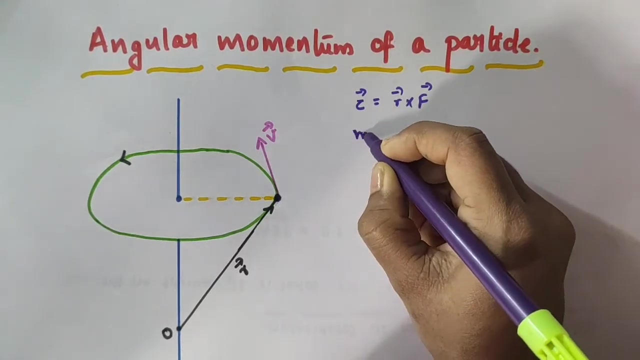 Torque was defined as it is actually the moment of a force. Okay. similarly, angular momentum can be referred to as moment of momentum or moment of linear momentum. Consider a particle. okay, consider a particle of mass. small letter m is moving with a velocity vector v along this path. 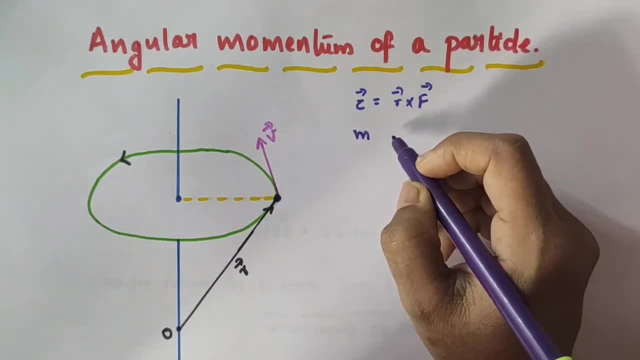 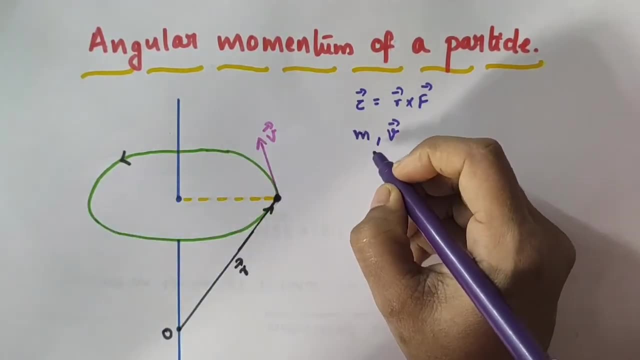 Okay, so it will have some momentum. no, that particle will have some momentum, because that particle has a mass m. It is moving with a velocity vector v along this path, So it will have some momentum. that momentum, linear momentum. that linear momentum will be what? 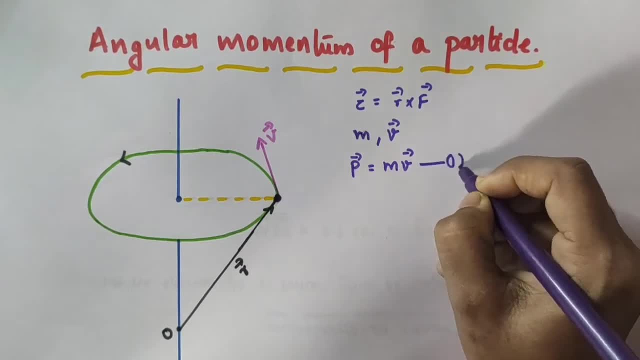 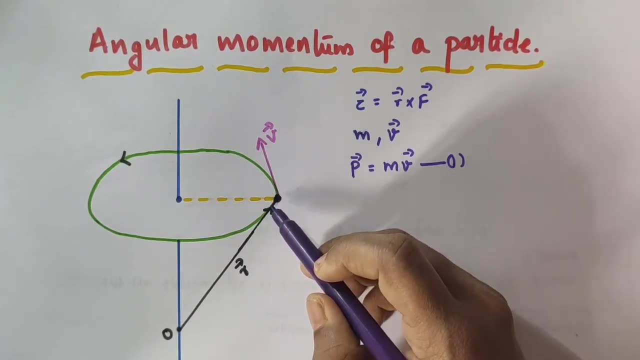 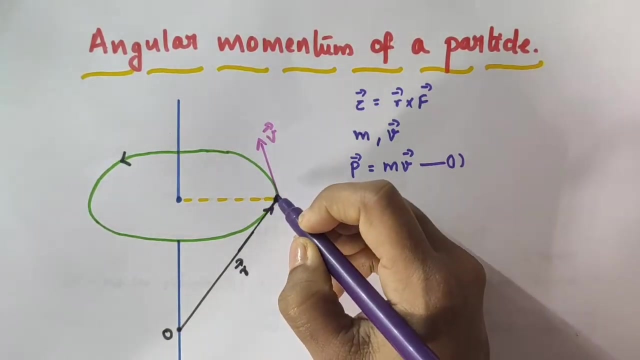 m into vector v. Okay, I am taking this as Equation number 1.. Now let vector r be the position vector of this particle with respect to or relative to the origin o. Okay, so you just imagine the particle is here. 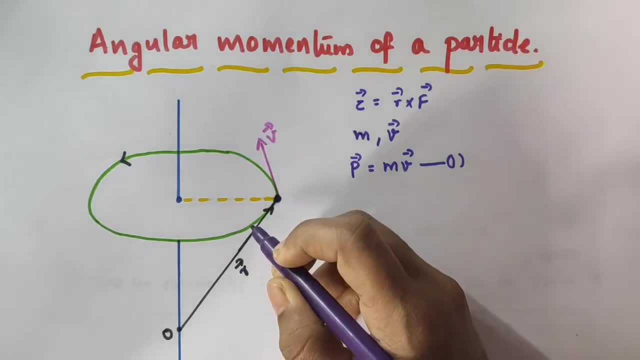 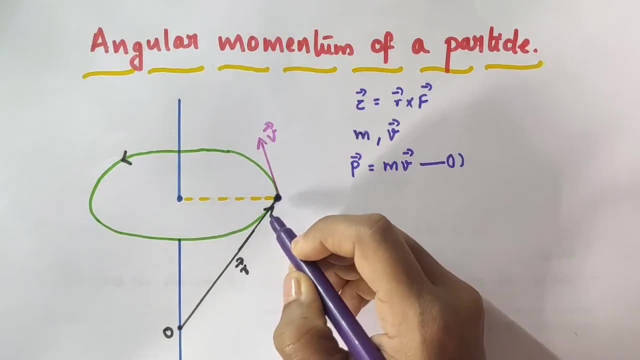 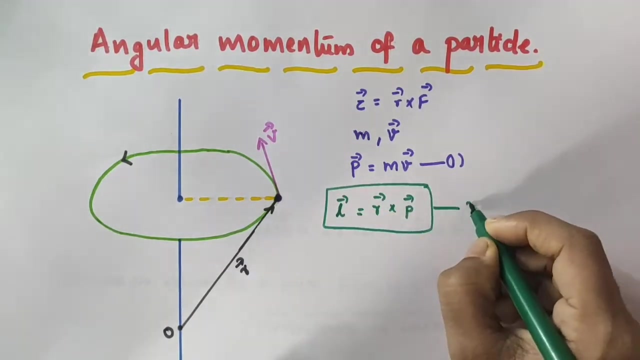 Then vector r is the position vector of this particle with respect to this origin o. The angular momentum of this particle with respect to this origin o is defined as: v. Vector l is equal to vector r cross vector p. Okay, and I am taking this as equation number 2.. 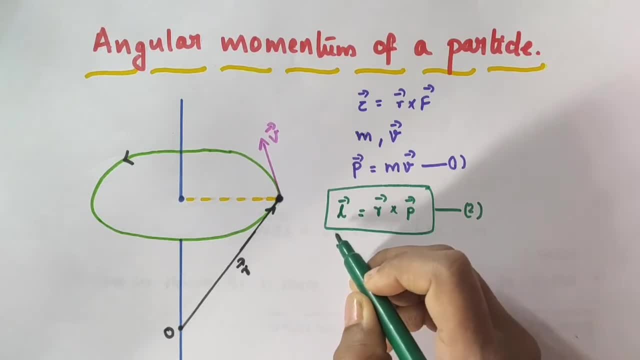 Where this vector l represents the angular momentum vector, because angular momentum is a vector quantity. Okay, vector l represents angular momentum, Vector p is actually the linear momentum vector and vector r is the position vector of this particle with respect to the origin o. Okay, now, while we have 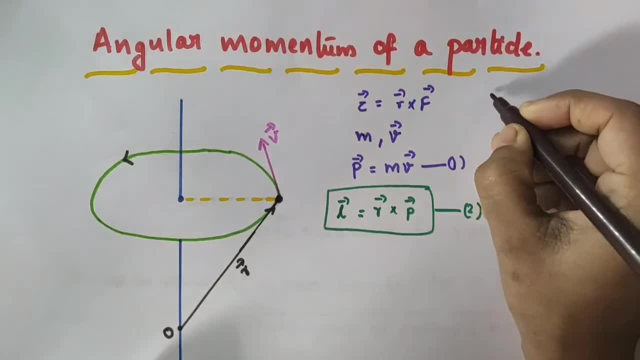 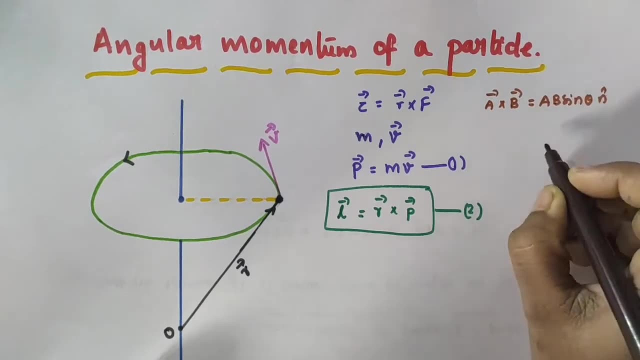 Discussed about the cross product, That is, vector a, cross vector b can be written as a into b, into sine of angle between them. Then n cap because vector product or cross product is a vector quantity. You know, okay, we have discussed about vector product in our previous video. 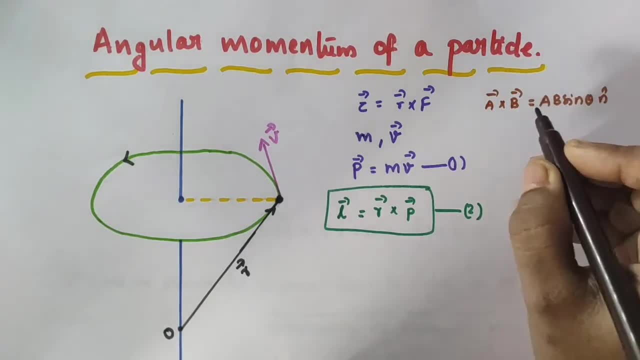 I will provide the link in the description box If you want you can watch that. Okay, anyway, vector a cross vector b is equal to a b sine theta n cap This a b sine theta is actually the magnitude of this vector product. 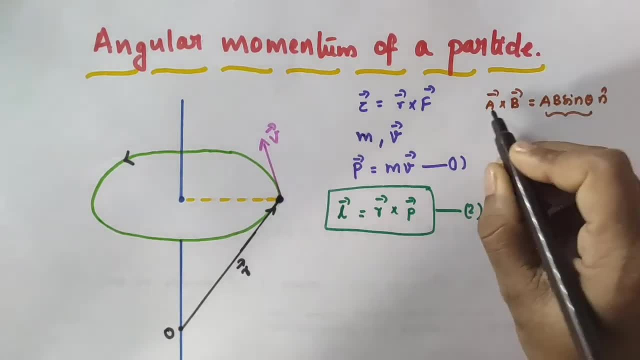 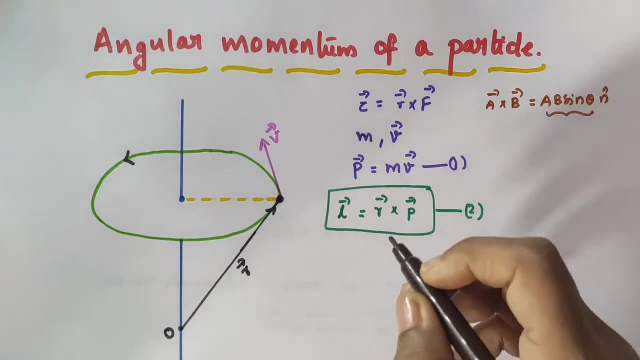 Okay, and n cap actually gives us the direction of this vector product. Alright. so, similarly, this equation that is vector l equal to vector r cross vector p. This can be written as: vector l is equal to r into p, into sine of angle between r and p. 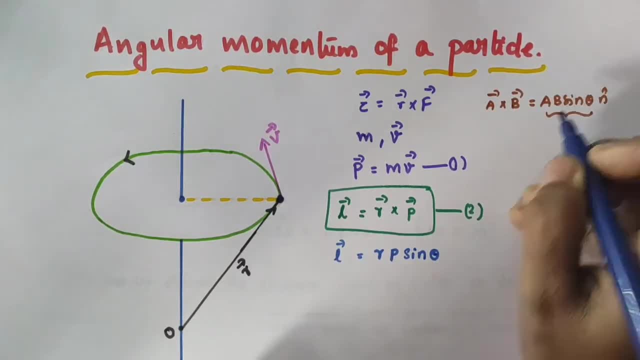 Okay, that is sine theta. vector a cross b equal to a b sine theta n cap. Similarly, vector l equal to r p, sine theta n cap. I am taking this As equation number 3.. Okay, where n cap is actually the unit vector which gives us the direction of this angular momentum, vector l: 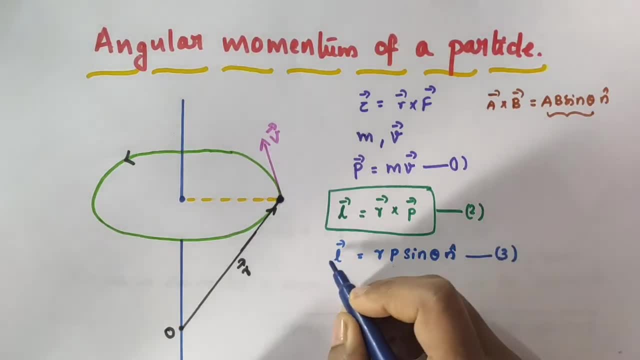 Okay, r p sine theta. that is the magnitude of this angular momentum. Okay, that is the magnitude of angular momentum. So I am simply writing it as l. Okay, I am not putting a vector sign here, because we are just taking the magnitude. 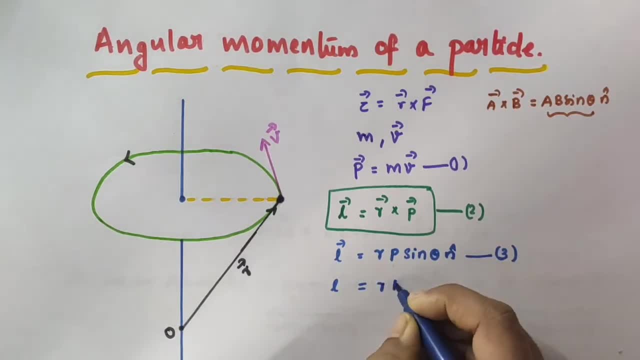 So magnitude of angular momentum is what r p sine theta. Okay, so this is the magnitude. So this is the magnitude of angular momentum: r p sine theta. I am taking this as equation number 4.. Okay, where this l is actually the magnitude of vector l. 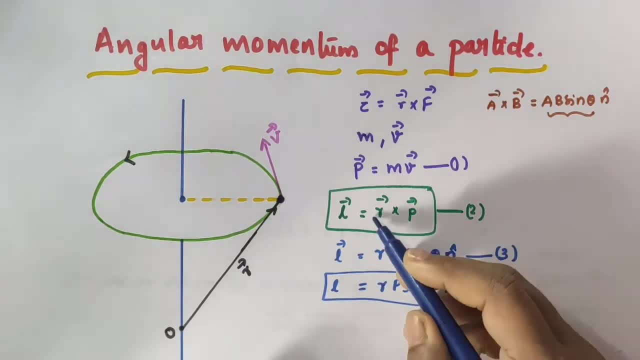 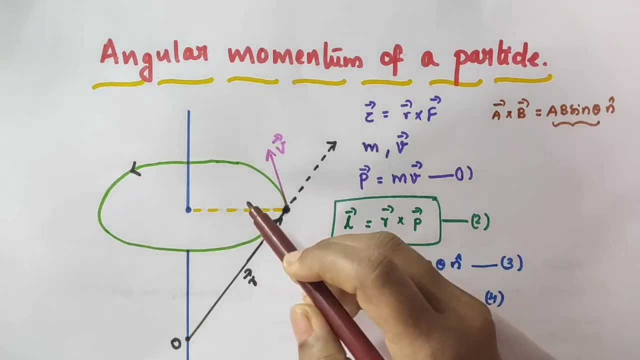 Magnitude of angular momentum. r is the magnitude of vector r, p is the magnitude of vector p. linear momentum, Then theta. it is actually the angle between vector r and vector p. Now let us consider this figure Here. actually, we said theta is actually. 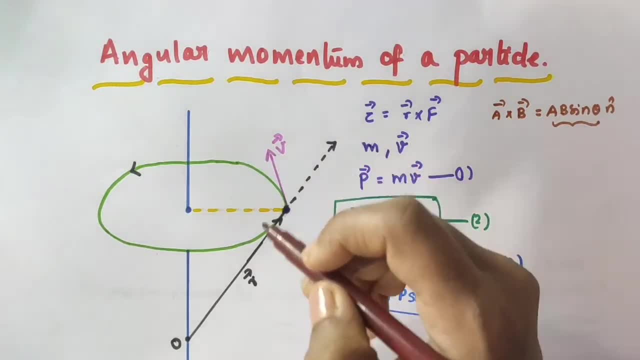 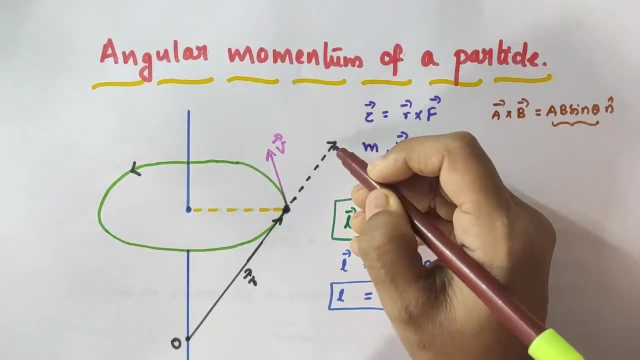 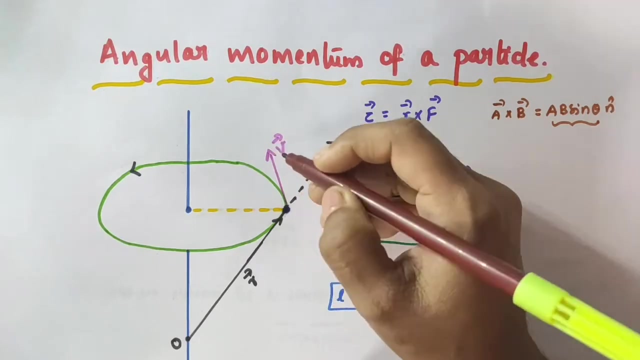 The angle between vector p and vector r. Now see, vector r is along this direction. I just extended the direction of vector r here by using dotted lines. No problem with that, because vector r lies along this direction. Okay, then see vector v. that is the velocity vector. 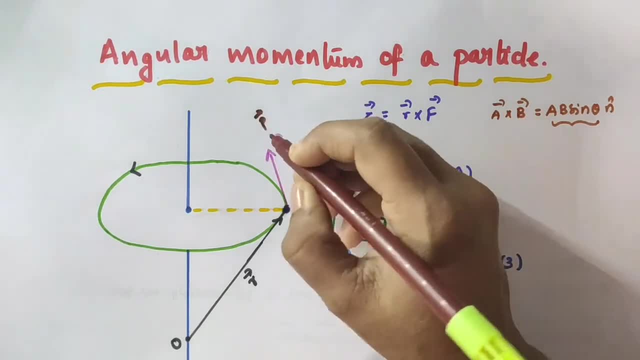 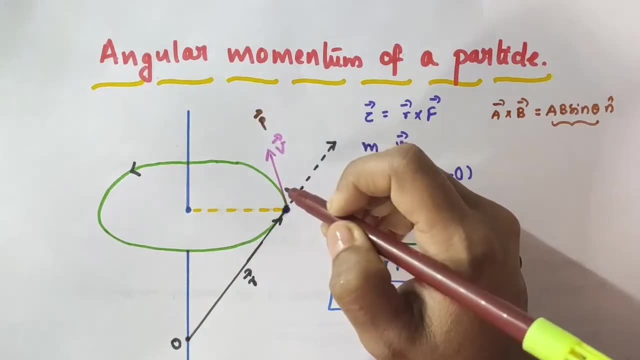 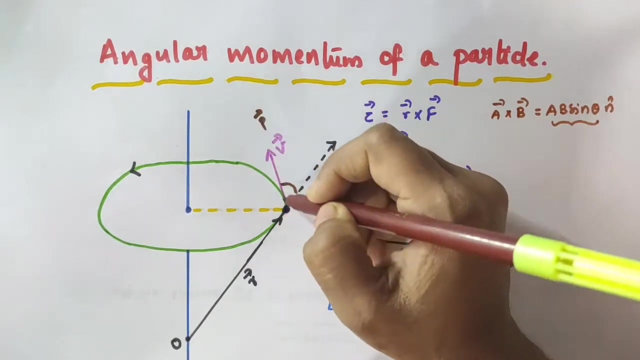 It is actually along this direction. So momentum vector, linear momentum vector p also will be along the same direction, Because vector p is equal to m into vector v, So momentum vector will also be along this direction. Alright, then theta is actually the angle between: this is vector r and this is vector p. 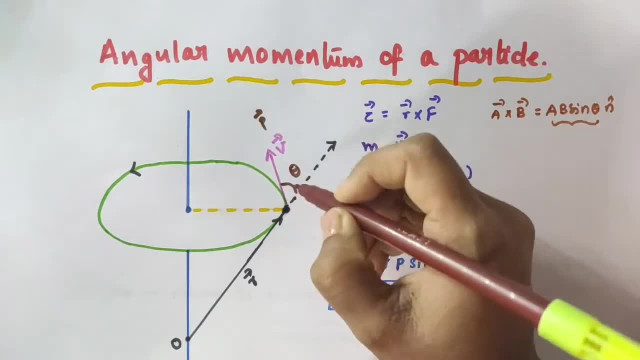 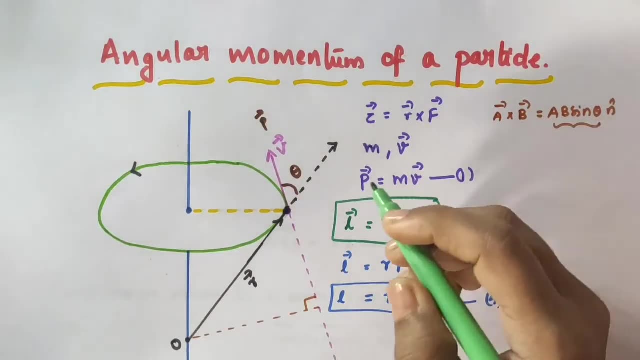 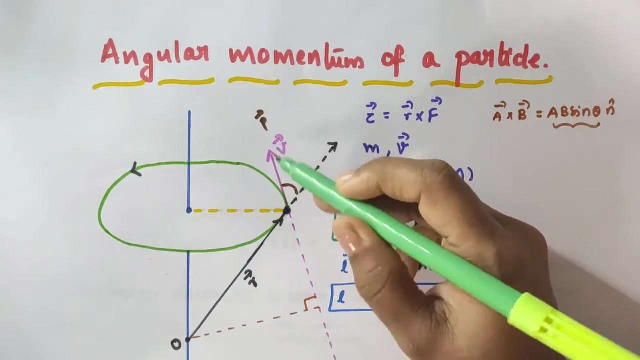 So theta is actually the angle between this vector r and vector p. That is, this angle is theta. Now, you see, I have just extended the line l. I mean, I have just extended this line of vector p, or momentum vector, using dotted line here. 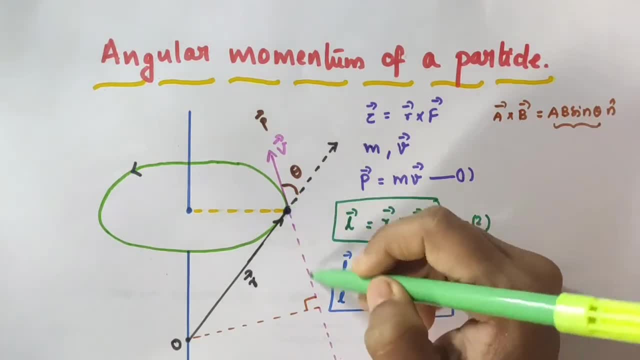 Okay, that is. This line is actually the line along which vector p lies. Okay, after that I just formed a triangle here. Okay, so that this angle is 90 degree. Alright, that is- I just joined this point- origin and the line where the vector p- momentum vector- lies. 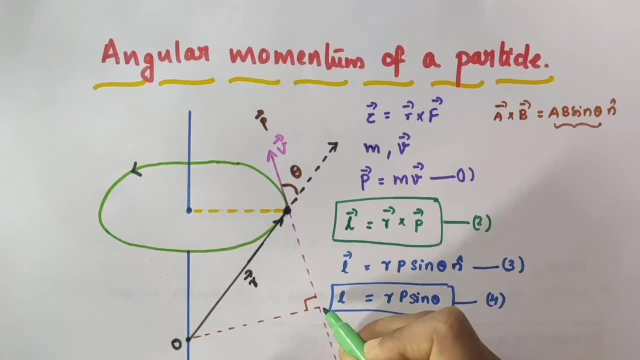 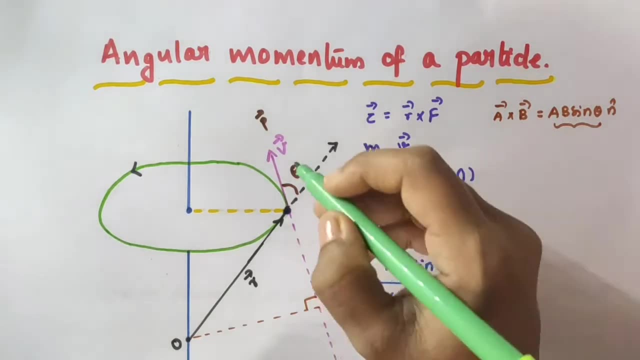 This pink dotted line and this origin by using this dotted line. I just joined them by using this dotted line. Okay, so that this angle, This angle, is 90 degree. Okay, now see, this angle is theta. So what about this angle? 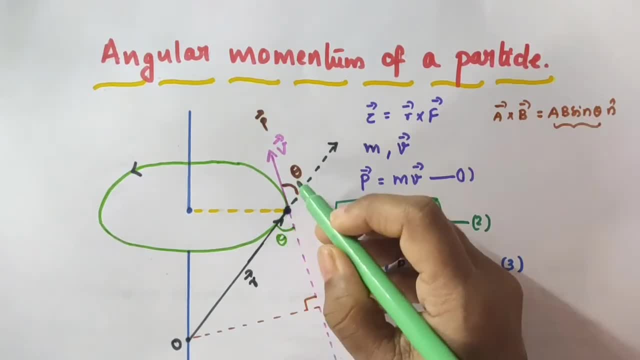 This angle also would be theta, Because opposite angles are the same. Okay, now if I am calculating sine theta here, What would be the answer? Sine theta. Okay, I am just considering this right angled triangle And I am just calculating sine theta. 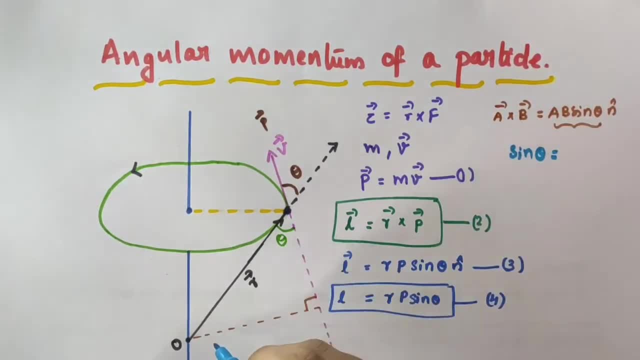 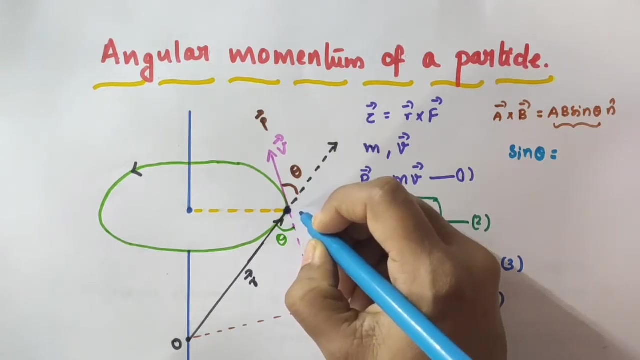 So sine theta is equal to opposite side. Opposite side means this side, Okay, Okay, divided by hypotenuse. So, okay, opposite side is this side. Okay, we can just name it as what. I am just taking this point as let. I am just taking this point as A, where the particle is. 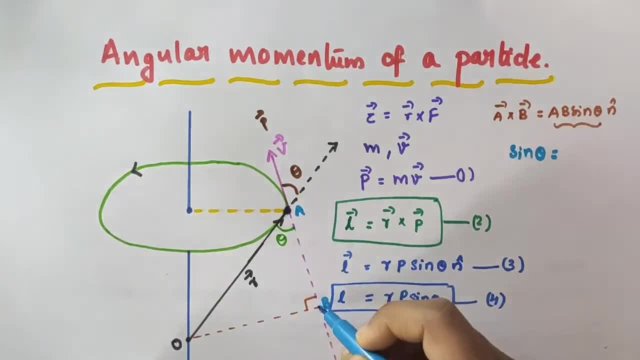 Then I am just taking this point as B. Okay, so triangle OAB. Okay, we are considering this. right angled triangle OAB. Okay, then here, sine theta is equal to opposite side. Opposite side means OB. Okay, divided by hypotenuse. 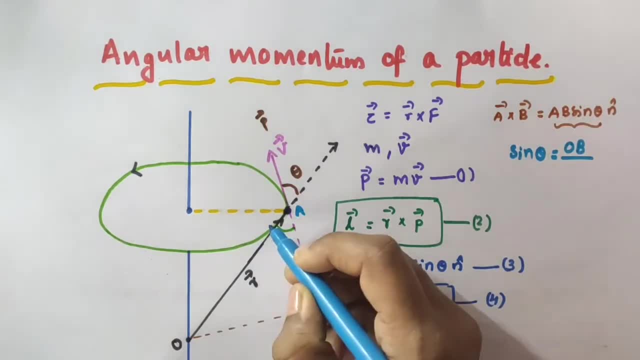 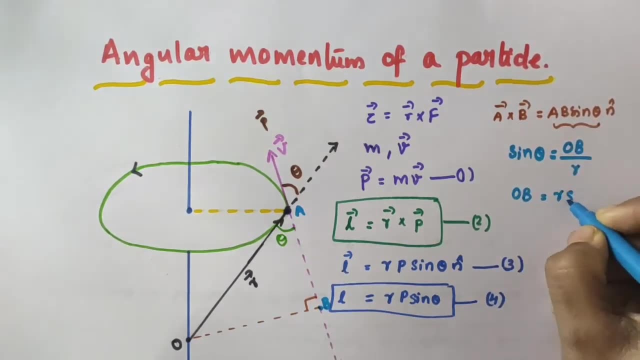 Hypotenuse means the side which is opposite to 90 degree, That is this side. It has a magnitude R. Okay, so OB divided by R, Alright, then OB is equal to what R into sine theta, That is, OB means this one. 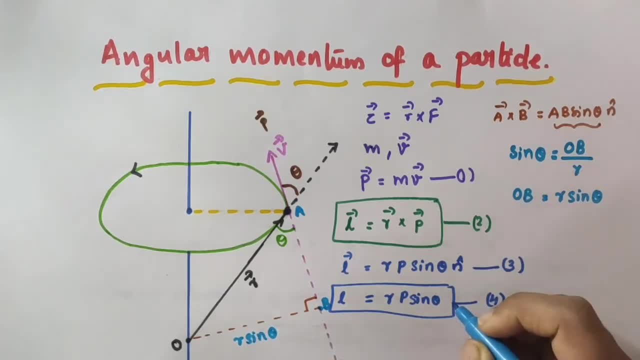 So this is actually equal to R sine theta. Okay, now you see this. R sine theta, It is actually the perpendicular distance of the directional line of vector P From the origin. Okay, that is, it is actually the perpendicular distance from the origin to the line of vector P. 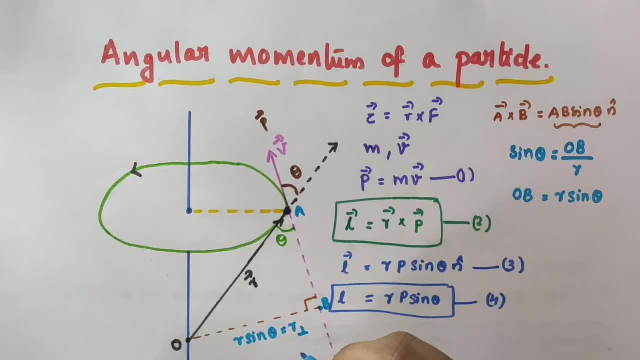 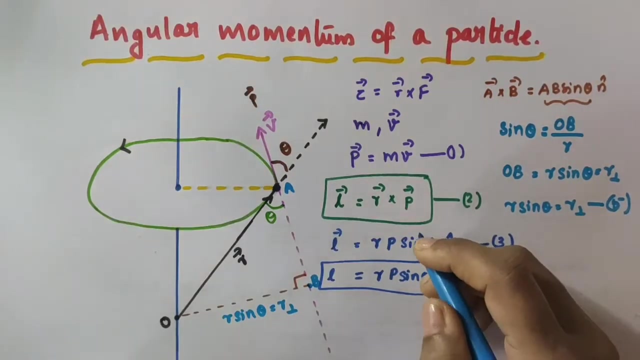 Okay, so I am taking this R sine theta as R perpendicular like this. Okay, this can be taken as R perpendicular. Alright, that is, R sine theta is equal to R perpendicular And I am taking this as equation number 5.. Next, you see, I am just forming a right angled triangle. 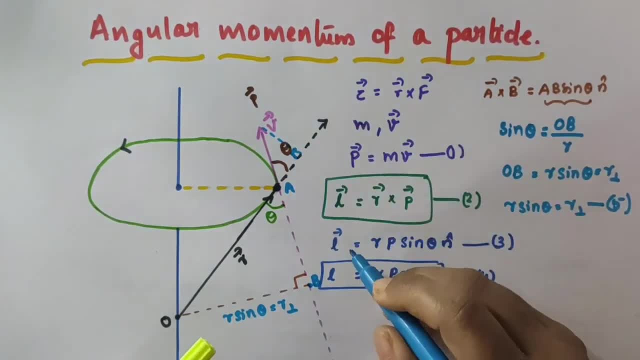 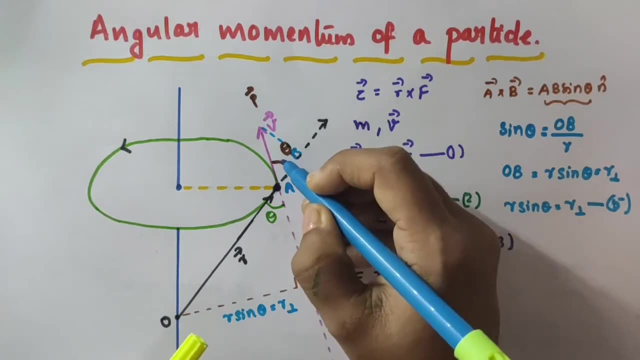 Triangle here. Okay, so that this angle is 90. See, this angle is theta. Okay, this is a right angled triangle. This angle is theta. So what about sine theta? Sine theta would be opposite side. Opposite side means this side. 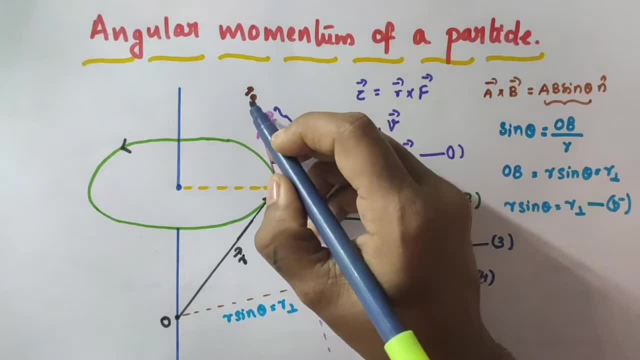 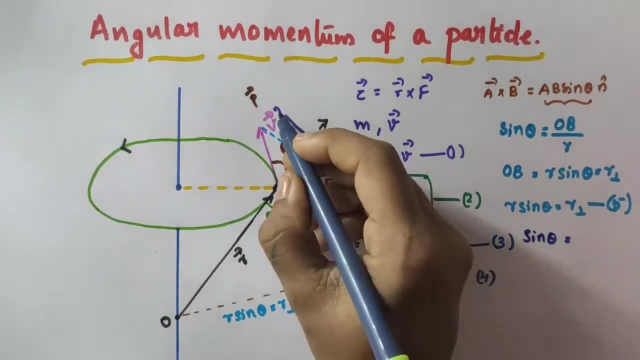 Divided by hypotenuse. Hypotenuse is this side which has a magnitude of momentum. Alright, so here, if you are calculating sine theta, we will get. sine theta is equal to opposite side, That is, this side Divided by 90.. 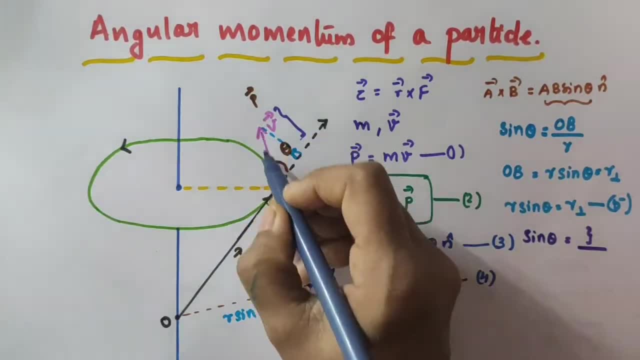 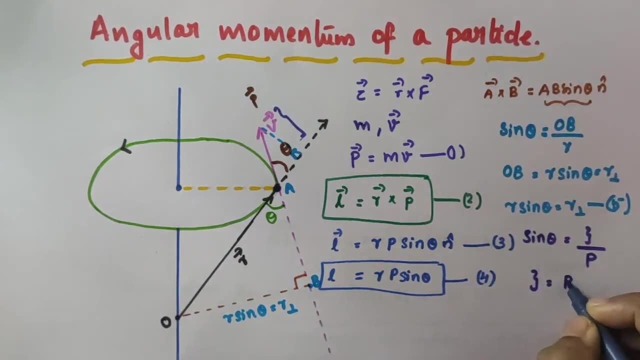 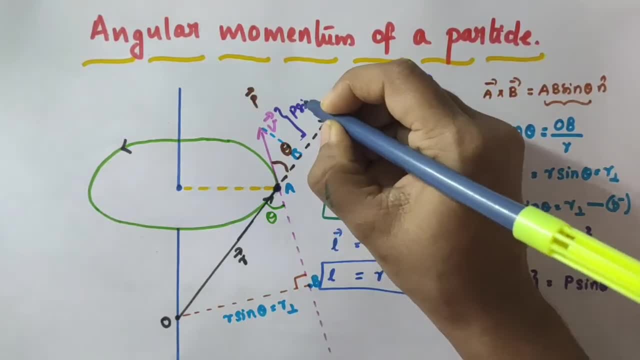 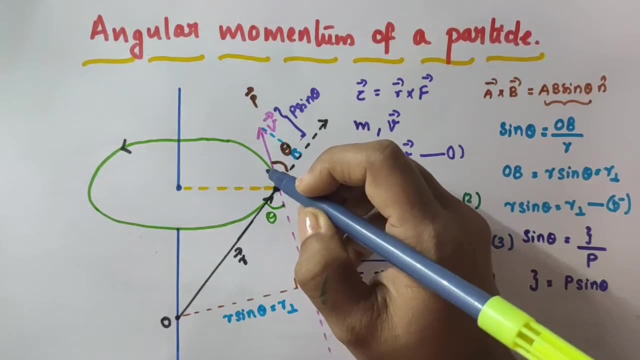 P sine theta. Okay, that is, this side will be equal to P sine theta. Okay, see this vector P can be resolved into two components. One is along the direction of vector R, Another one is perpendicular to the direction of vector R. 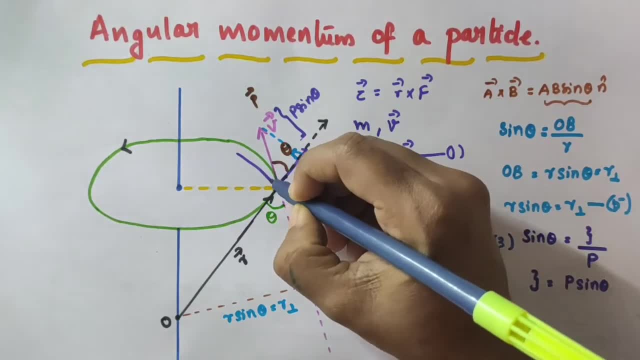 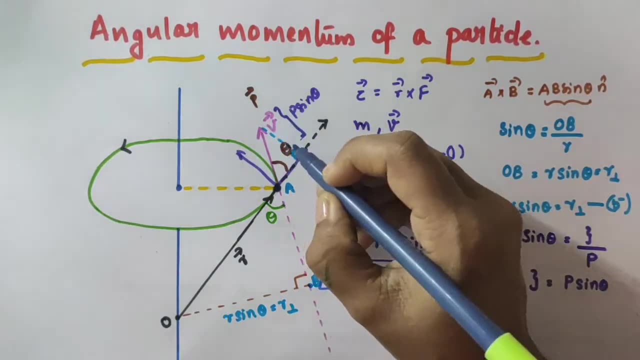 Okay, we can resolve this vector P into two components. One is along the direction of vector R, Another one is perpendicular to vector R. Okay, so here, P sine theta. You see, this is P sine theta. That is actually parallel to this vertical component. 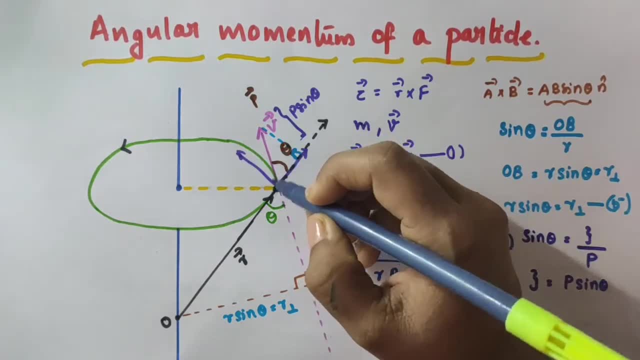 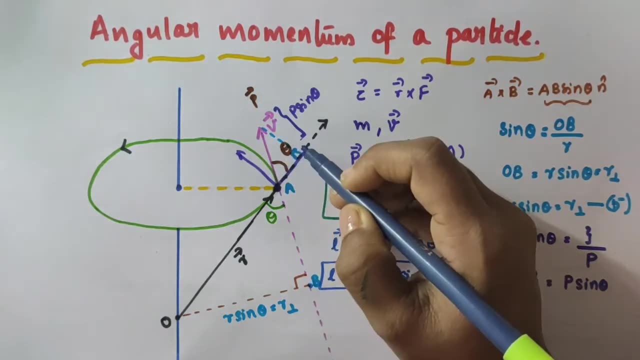 That means both are equal. Okay, both will have the same magnitude. So P sine theta is actually the component of vector P perpendicular to this. Okay, that is, P sine theta is actually the component of vector P in a direction perpendicular to vector R. 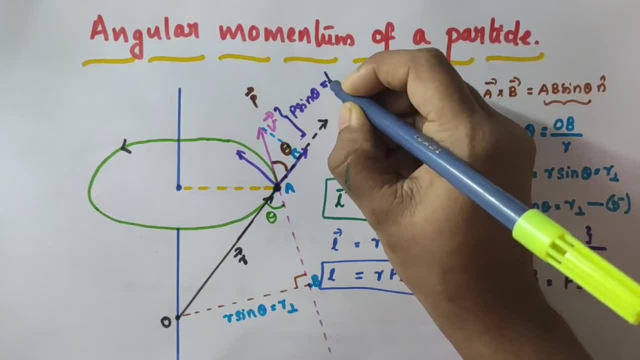 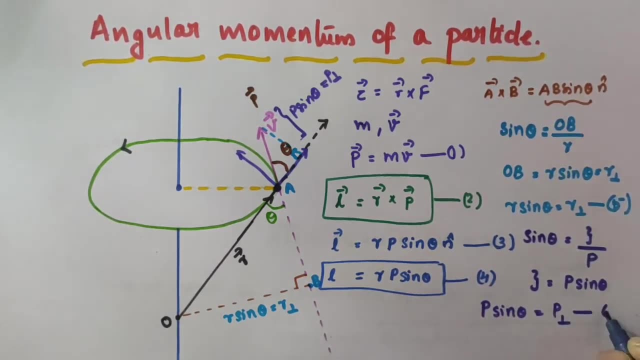 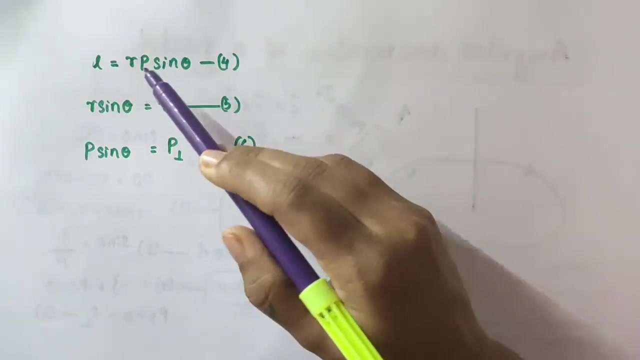 Okay, So I am writing this P sine theta as P perpendicular. Alright, we are writing P sine theta as P perpendicular And I am taking this as equation number 6.. So you see, we have equation number 4, as L is equal to R P sine theta. 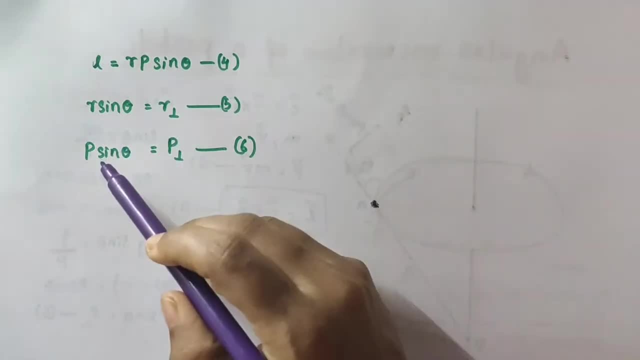 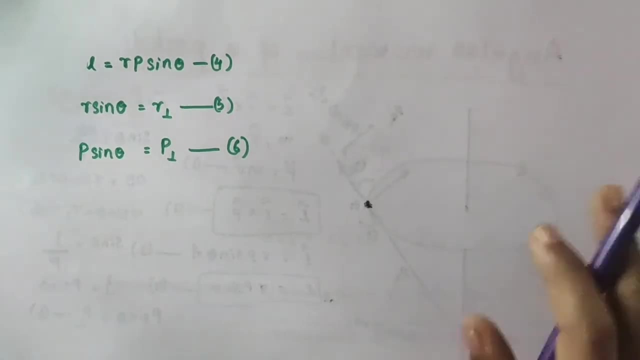 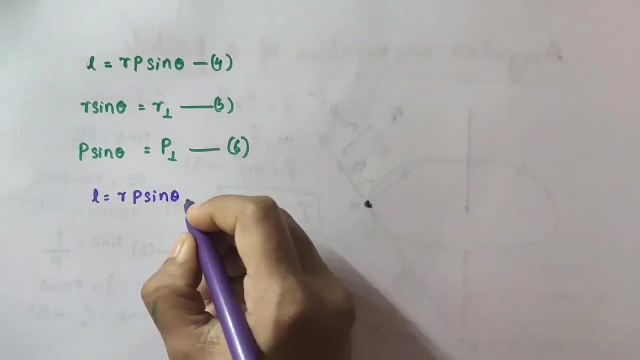 Then equation number 5 is R sine theta equal to R perpendicular. Equation number 6 is P sine theta is equal to P perpendicular. Alright now, So I am taking this equation L equal to R P sine theta, This equation number 4 can be written as what: 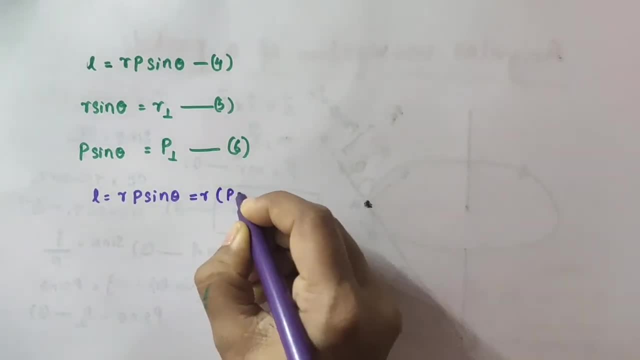 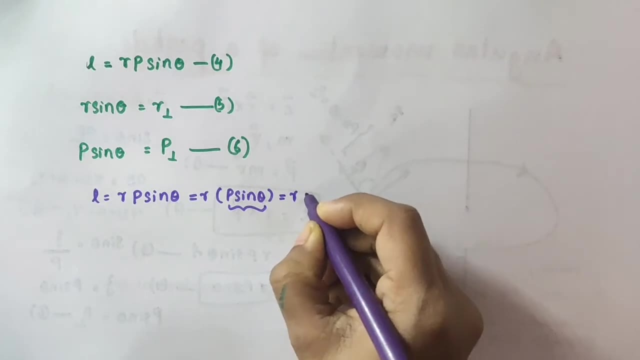 This R, P sine theta, that can be written as R into P sine theta. No, Okay now what is this P sine theta? P perpendicular, So this can be written as R into P perpendicular. Alright, so the magnitude of angular momentum can be written as R into P perpendicular. 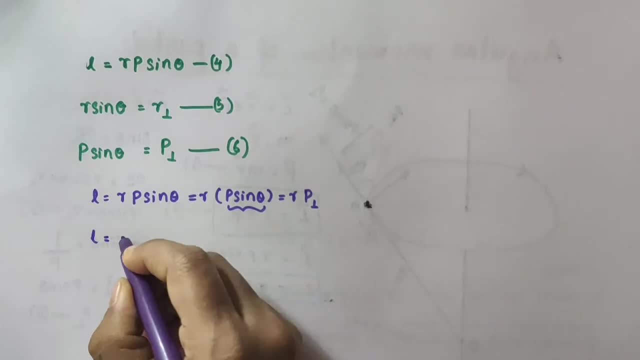 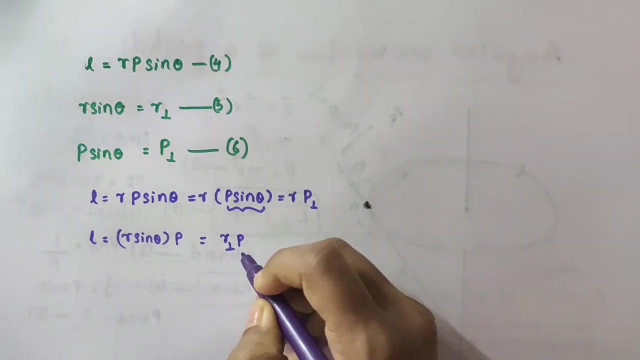 Alright, similarly, Similarly, this equation, R, P sine theta Can be written as R into sine theta, then into P. Okay, what is this? R into sine theta? This is R perpendicular, So R perpendicular into P. Okay, so magnitude of angular momentum can be written as R perpendicular into P. 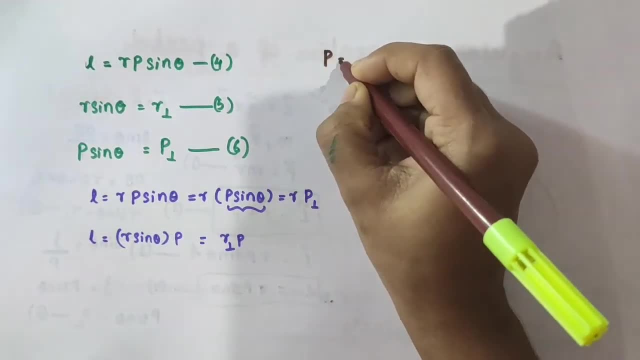 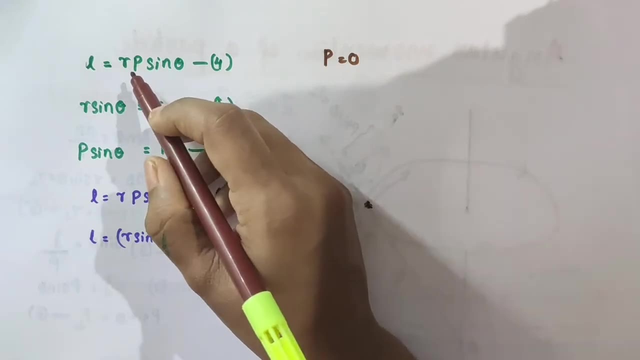 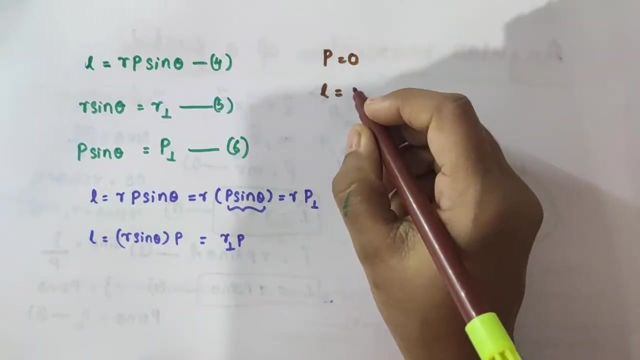 Now if linear momentum P equal to 0.. What about the magnitude of angular momentum? Magnitude of angular momentum is L equal to R, P sine theta. So magnitude of angular momentum becomes R into 0, into sine theta. So 0 into any value, will give you 0.. 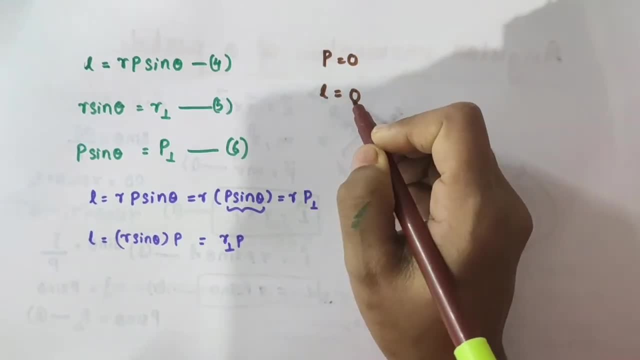 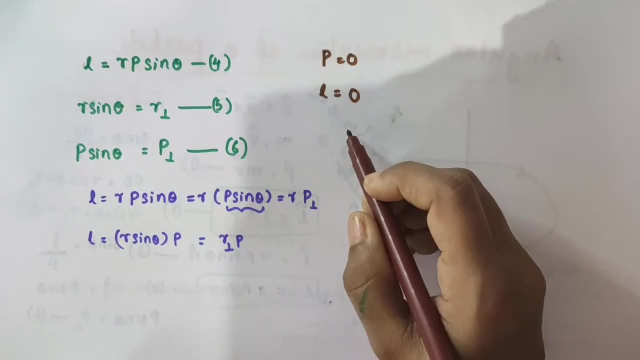 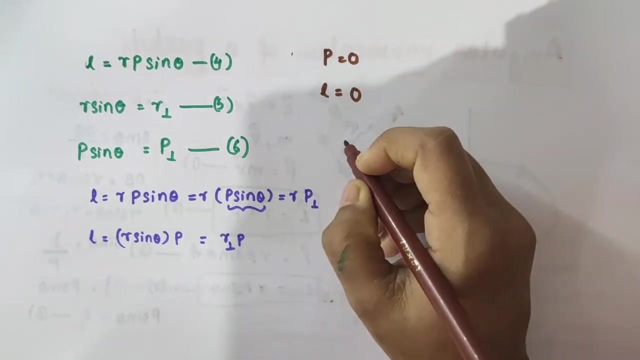 Okay, that is the magnitude of angular momentum becomes 0.. If the linear momentum vanishes, that is, becomes 0.. Okay, now What if the particles at the origin? If the particles at the origin, then R equal to 0.. 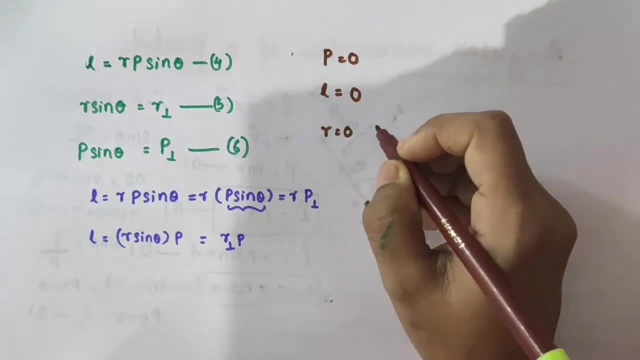 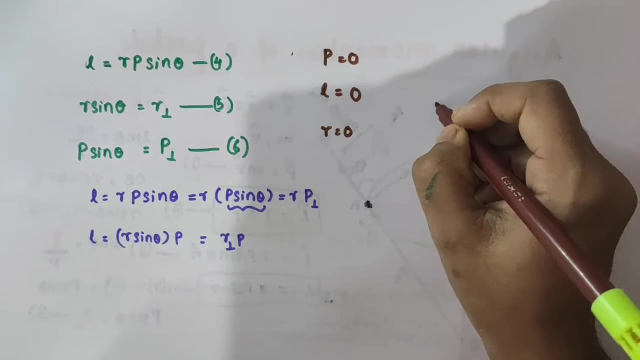 No, Okay, Because R is actually the distance from the origin to the point where the particle is. So when the particle is at the origin, no distance between the origin and that point. See, if this is the origin and the particle is somewhere here. 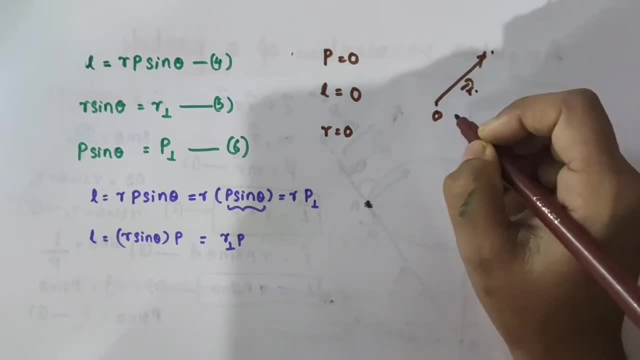 Alright, So this distance that is actually taken as a position vector, vector R. Its magnitude is R. Okay, Now, if the particle is at the origin, then there is no distance between that particle. I mean, there is no distance between the origin and the position of that particle. 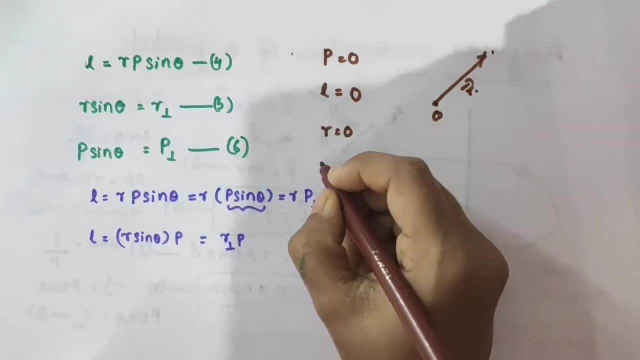 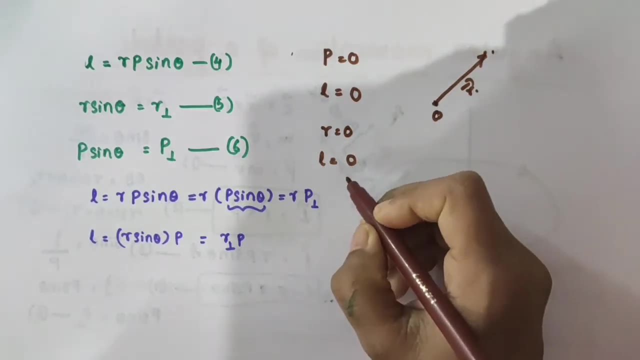 Okay, Then R becomes 0. So when R equal to 0, the magnitude of angular momentum that becomes 0 into any value will give us 0. Okay, That is. magnitude of angular momentum becomes 0 if the particle is at the origin. 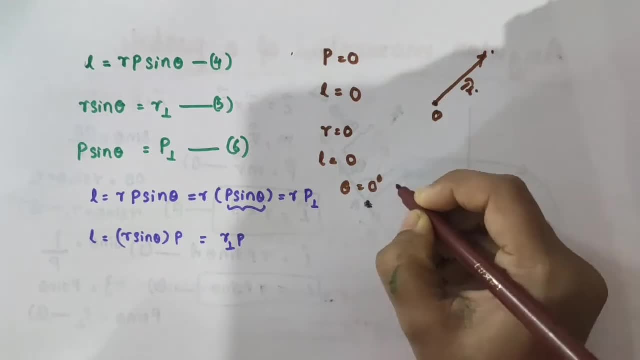 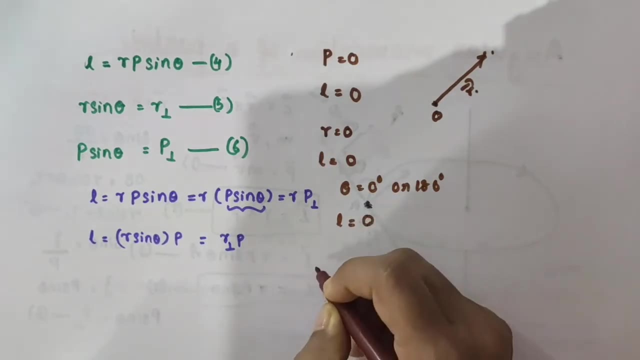 Okay. Next, if theta equal to 0 degree or 180 degree, what happens to the magnitude of angular momentum That becomes 0. Why? Because sine 0 is 0. Sine 180 is equal to 0. Okay. 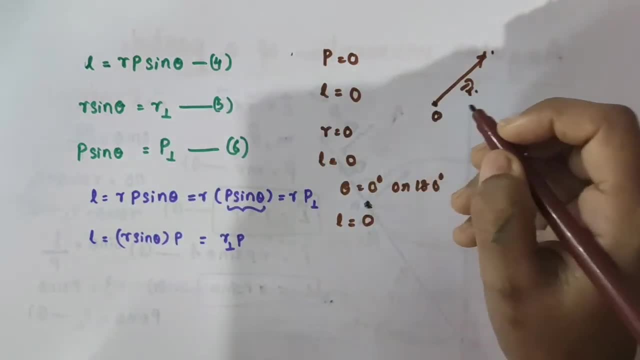 Okay, Theta equal to 0 or 180 means the directional line of vector P that passes through the origin, either along the same direction of vector P or opposite to the direction of vector P. Okay, In such a case, angular momentum becomes 0.. 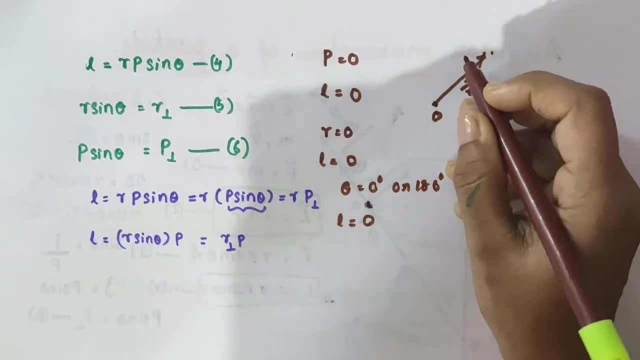 I mean here vector P. sometimes it will be along the same direction of vector R and sometimes opposite to the direction of vector R, So that case theta will be equal to 0 or 180.. Okay, Then in such a case angular momentum becomes 0. 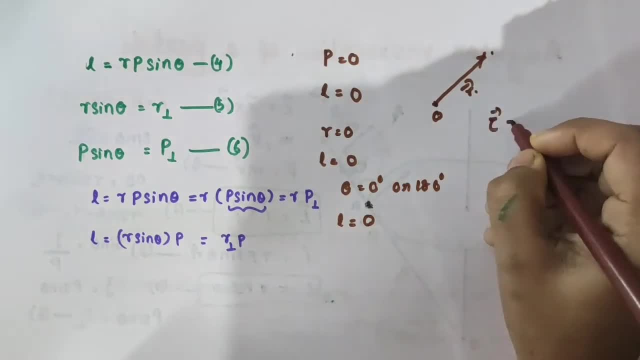 Okay, So you see, torque, it is actually the moment of a force and it is defined as vector R cross vector F and angular momentum. it is actually the moment of linear momentum and it is defined as vector R cross vector P. Torque is actually moment of force, defined as vector R cross. 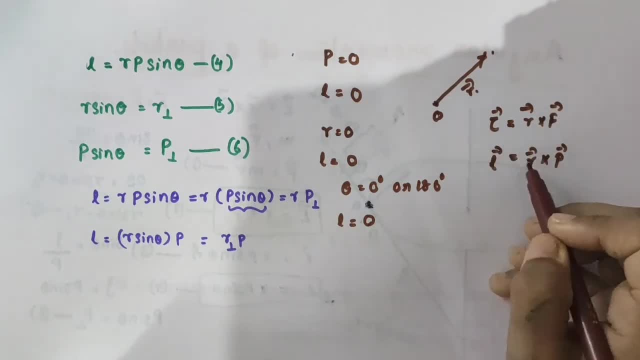 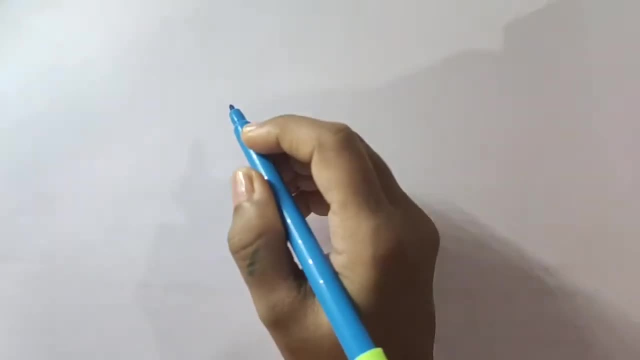 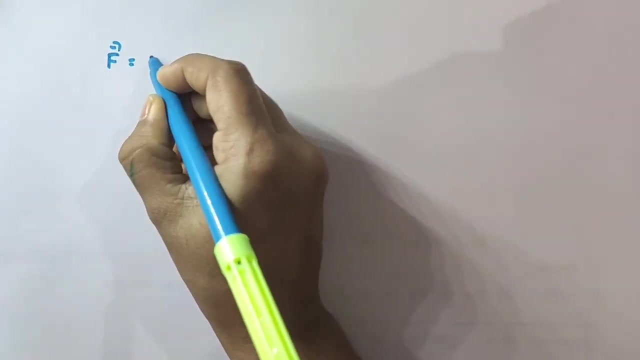 vector F, Angular momentum is actually the moment of linear momentum. So vector R cross vector P. Now see, we have from Newton's second law of motion. for the translational motion of a single particle, vector F is equal to d, vector P divided by dt. 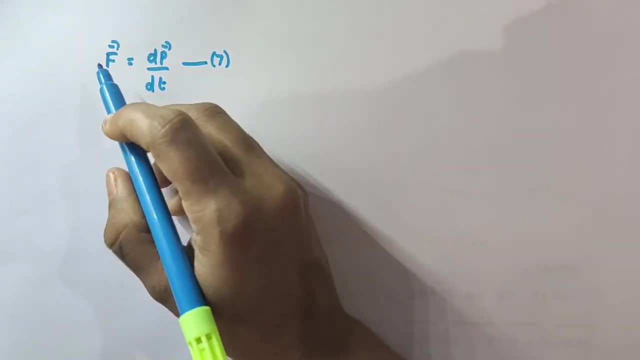 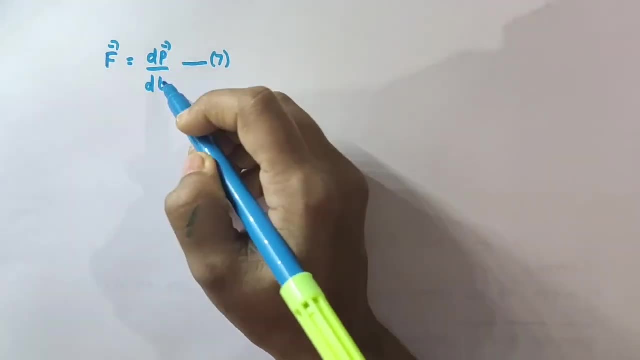 I am taking this as equation number 7,, that is, we have the force as the rate of change of vector P. Vector P is the moment of, so we have the force as the rate of change of momentum. This expression actually gives us a relation between force and linear momentum in translational. 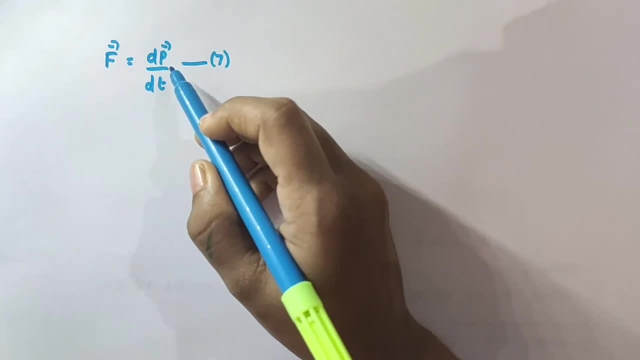 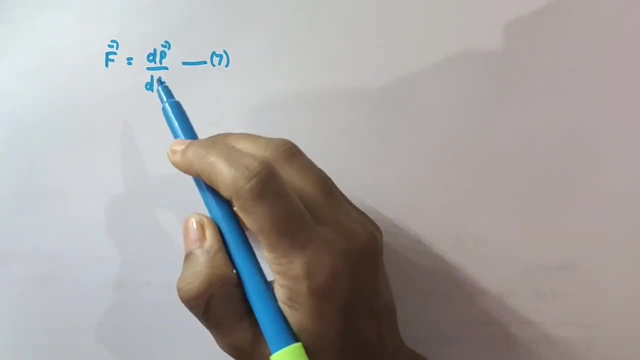 motion of a, in the case of translational motion of a single particle. Okay, Let us try to obtain the rotational analog of this equation. That is, we are trying to get the rotational analog of the relation between force and linear momentum of a particle. 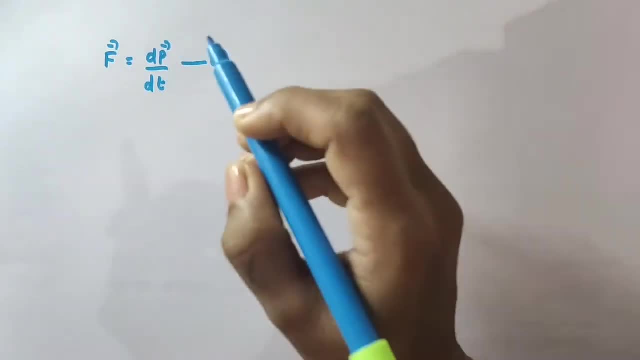 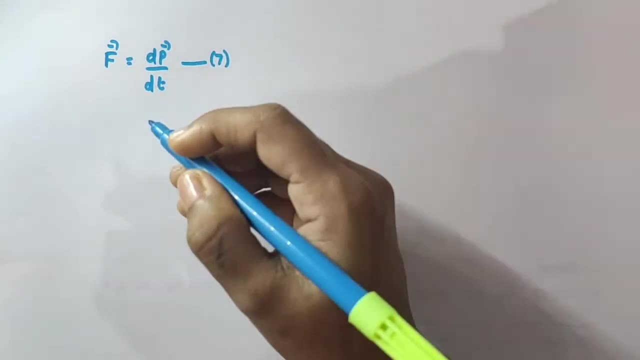 That is the relation between moment of force or torque, and angular momentum. Okay, We are trying to obtain the rotational analog of this relation. That is, we are trying to obtain a relation between moment of force- that is torque- and angular momentum. moment of momentum that is angular momentum. 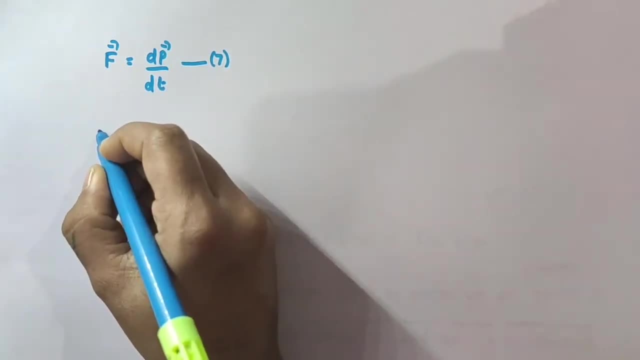 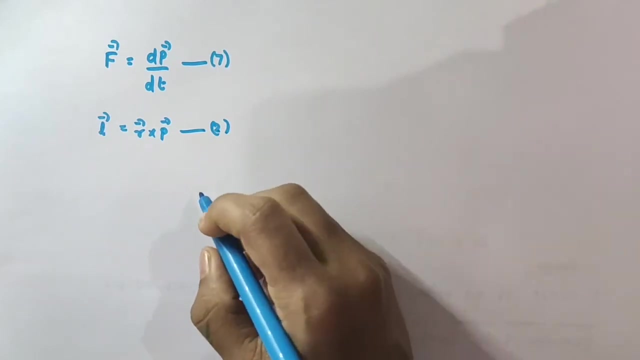 Okay, So for that, let us consider this equation: for angular momentum, vector L is equal to vector R cross vector P. This was actually equation number 2.. I hope you remember this. Okay, Now I am going to differentiate this equation. 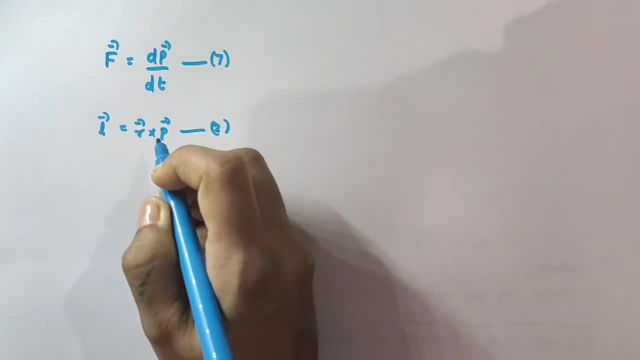 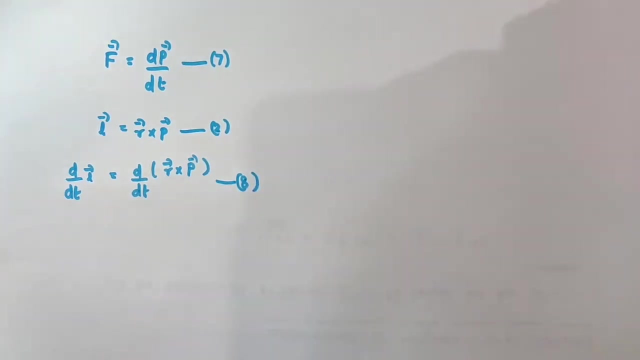 I am going to differentiate both sides. I am going to differentiate both sides of this equation with respect to time. So this becomes: d by dt of vector L is equal to d by dt of vector R cross vector P. Okay, I am taking this as equation number 8.. 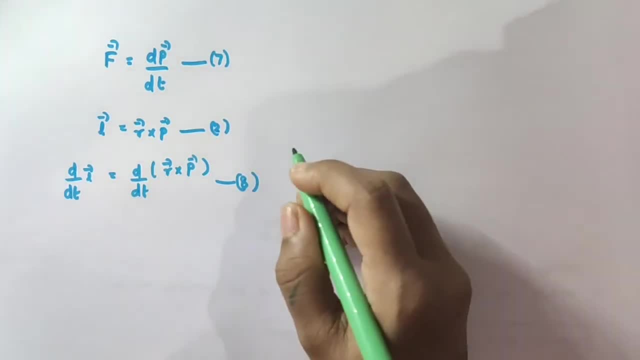 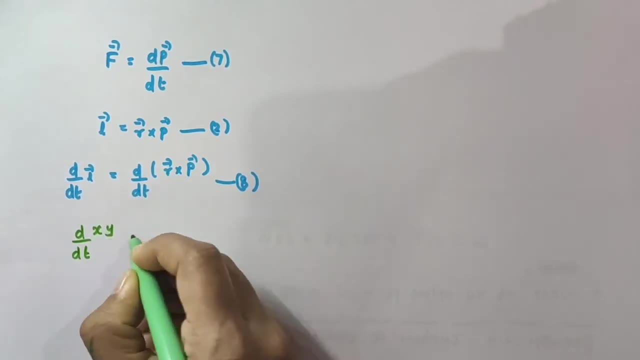 Alright, Now you see what is the product rule for differentiation. The product rule for differentiation is d by dt of x into y is equal to. this is the first one. This is the first function. This is the second function. First function, that is, x into the derivative of the second. 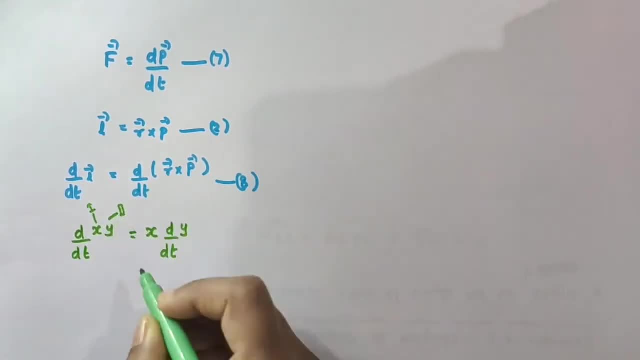 Second is this: Okay, This is the first function and this is the second function. So the product rule is the first function into derivative of the second, plus second into derivative of the first. Okay, So let us apply this product rule for differentiation to the right hand side of this equation 8.. 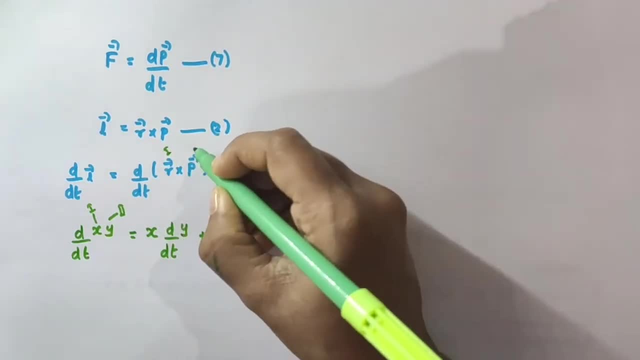 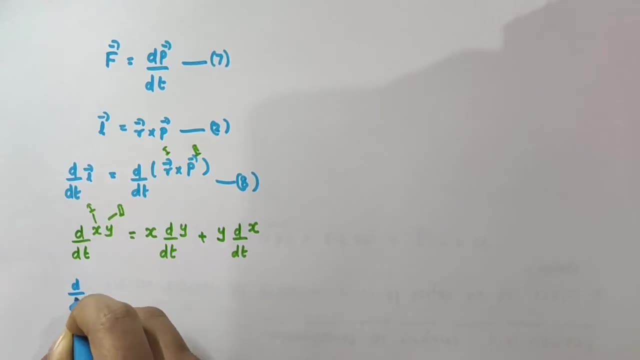 Okay, So here you see vector R. So vector R is the first function and vector P is the second function. Alright, So this equation becomes: what d by dt of vector L is equal to first function, into derivative of the second. 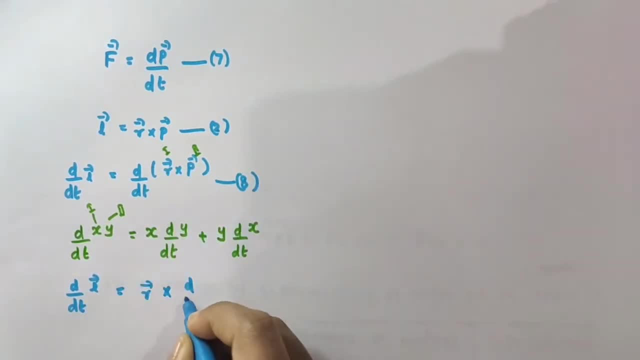 So vector R cross. this is cross product. So vector R cross. d by dt of vector P. Okay, Plus second into second, one is vector P, Then into here, it is cross product. So cross, Then derivative of d by dt of. 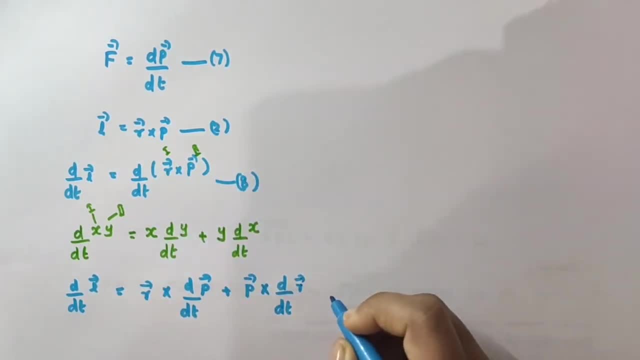 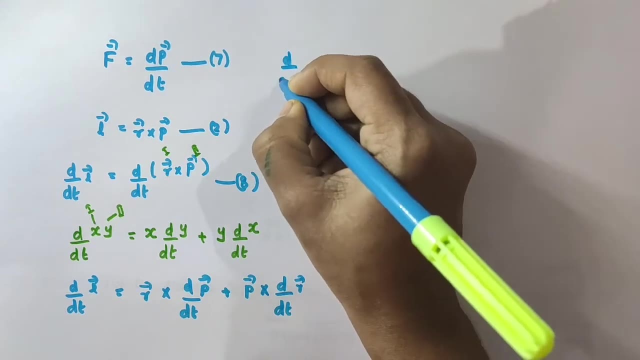 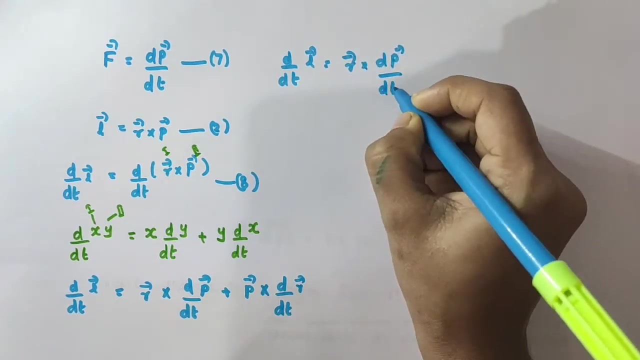 The first one. First one is vector R. Okay, So this equation can be written as: d by dt of vector L is equal to vector R cross d. vector P divided by dt. Okay, Plus this vector P, it is actually the linear momentum vector. 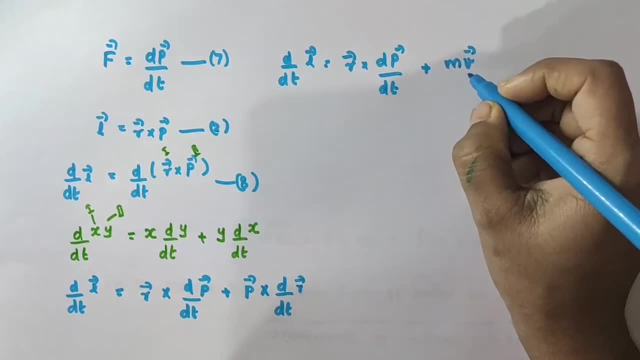 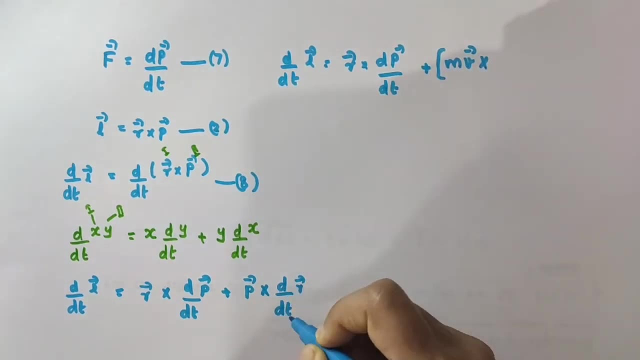 No, So that can be written as m into vector V, because vector P is equal to m into vector V. Okay, Then cross Cross D by dt of vector R. What is d by dt of vector R? It is actually the derivative of the position. no. 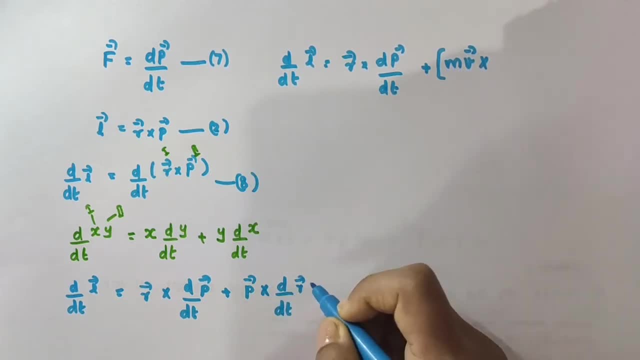 Derivative of displacement or derivative of position vector, That will give us velocity vector. So that will be vector V. Okay. Derivative of vector R, that is actually equal to vector V, velocity vector. Okay, Now you see, here we have m into vector V, cross vector V. 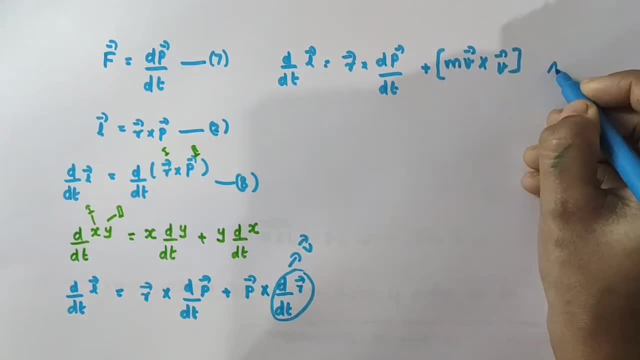 Vector V: cross vector V. What will be its answer? See vector A. cross vector A is equal to n Null vector. Okay, This we have discussed. while we have discussed about the vector product or cross product, I will provide the link in the description box. 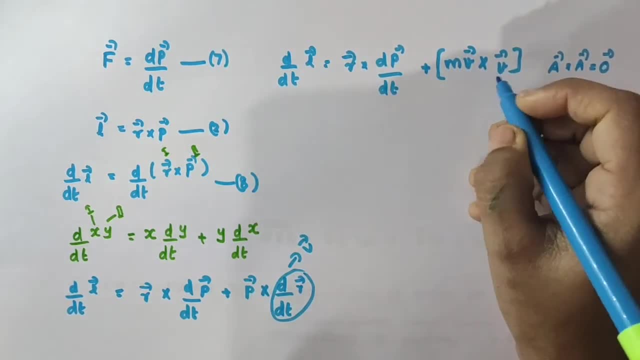 If you want, you can watch that. Okay. So here, vector V cross vector V. that will be equal to what? That will be equal to 0.. Its magnitude will be 0.. It will be a null vector. Its magnitude will be 0. 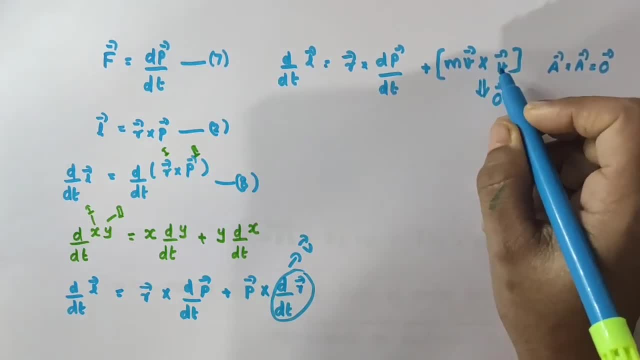 Because vector V and vector V, you know so they are parallel. So vector product vanishes, because theta becomes 0. Okay, What is sine 0?? Because vector V cross vector V means V into V, into Sine of angle between them. 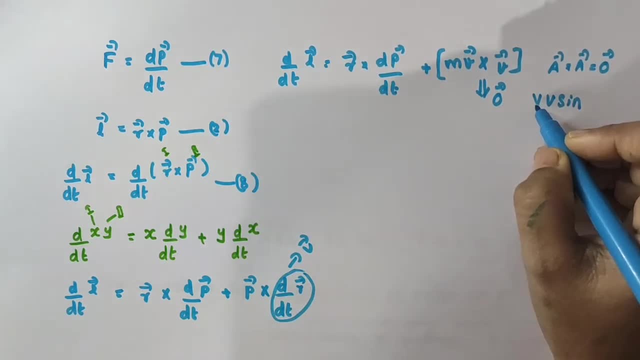 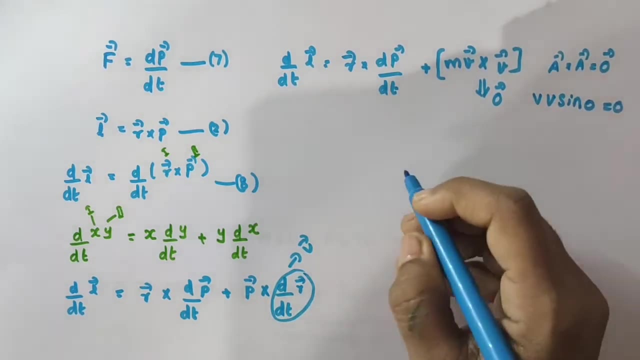 Both are V. you know Both are along the same direction. no, Both are parallel. no, Okay, So angle between them is 0.. Sine 0 is 0. So this becomes 0.. Okay, So we have d by dt of vector. L is equal to what? 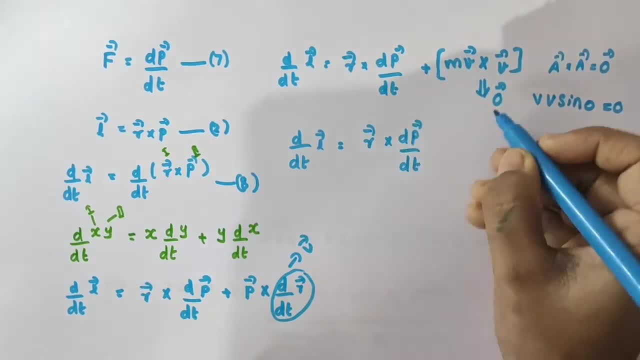 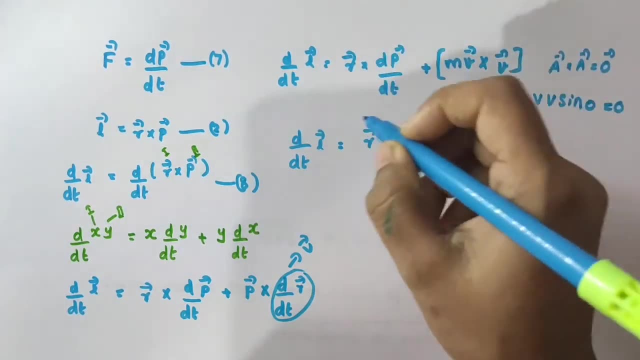 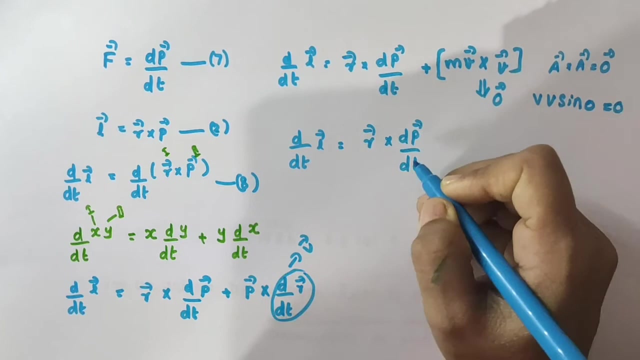 Vector R cross d vector P divided by dt, This becomes a null vector. Null vector plus any value. I mean anything that will give you that value, Nothing itself. Okay, So we can write: vector d by dt of vector L is equal to vector R cross d vector P divided by dt. 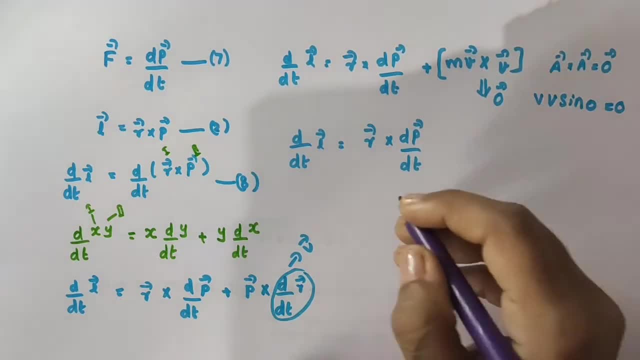 Alright, Now you see what is this. vector R, cross vector, I mean d vector P divided by dt. This has become like this: no, Okay, So d by dt of vector R cross vector P has become vector R cross vector, I mean d vector P divided by dt. 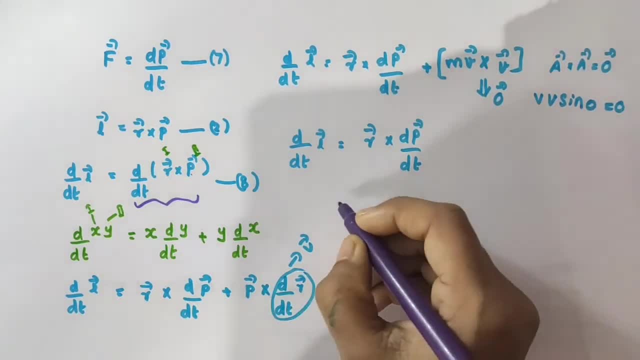 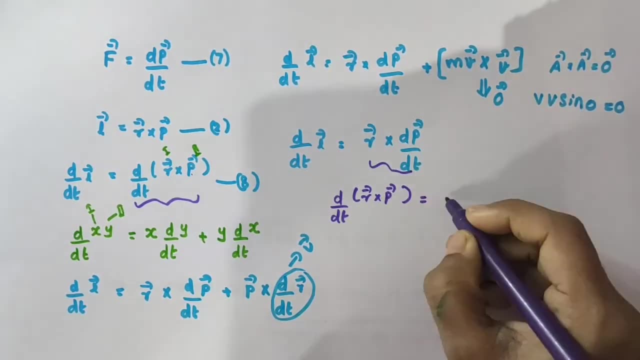 While we apply the product rule for differentiation. Okay, That is actually this: d by dt of vector R cross vector P. That is actually what This one, That is, vector R cross d vector P divided by dt. Alright, I am taking this as equation number 9.. 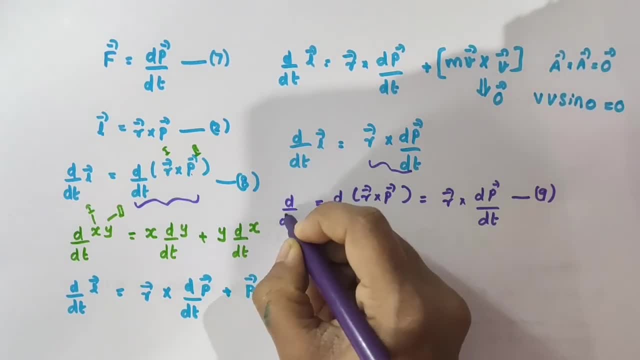 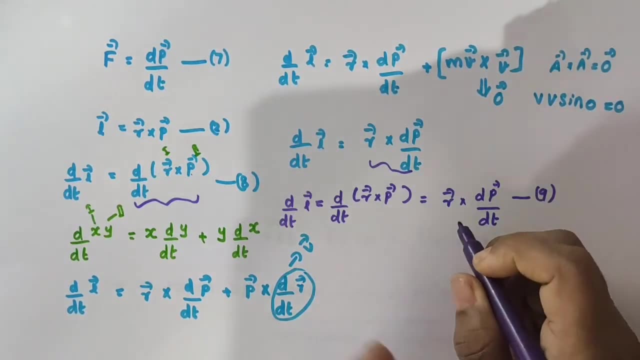 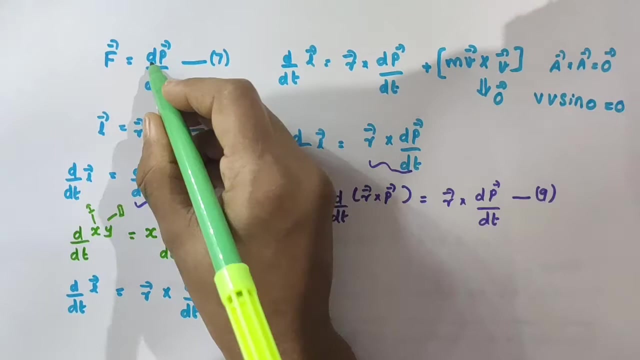 Okay, This is equal to d by dt. of vector L. Okay, Both are the. I mean all the three are the same. I mean have equal value, Alright. Alright Now from equation 7, we have: vector F is equal to d. vector P divided by dt. 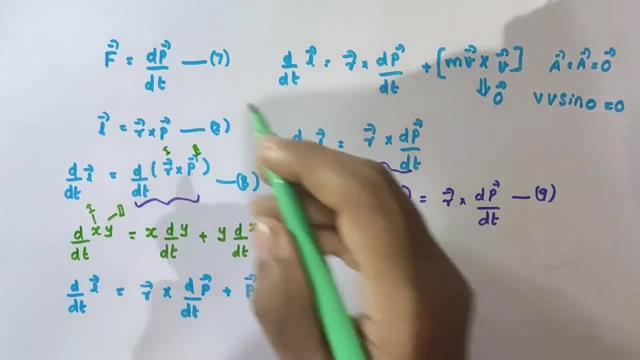 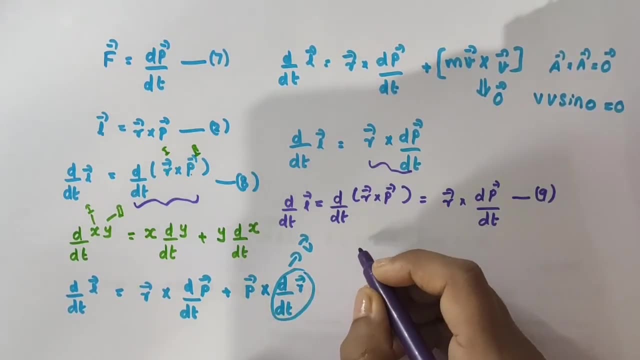 Okay, Now I am going to substitute this equation number 7 in equation number 9.. Alright, So this equation number 9 becomes what? Equation number 9 becomes? d by dt of vector L, which is equal to d by dt of vector R cross vector P. 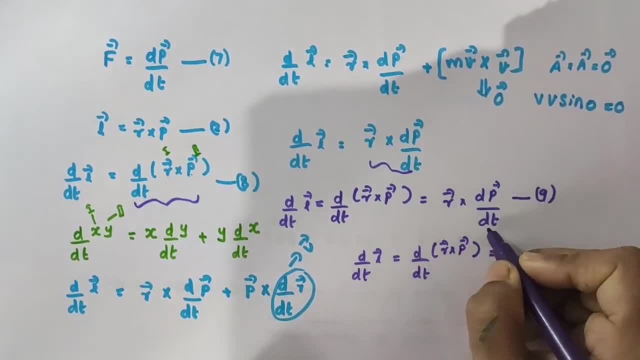 This is equal to what Vector R cross d vector P. This is equal to vector R cross d vector P divided by dt. What is this? d vector P divided by dt? That is vector F. So vector R cross vector F. Okay. 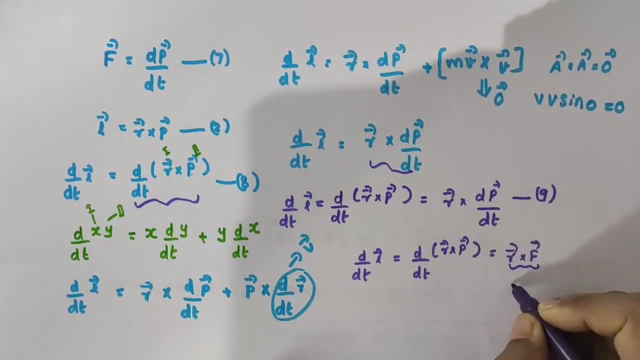 Now you see what is this? vector R cross vector F. Vector R cross vector F is vector tau. no, Okay, This is the. I mean torque. no, Alright, Torque is defined as vector R cross vector F, So this is actually the torque. 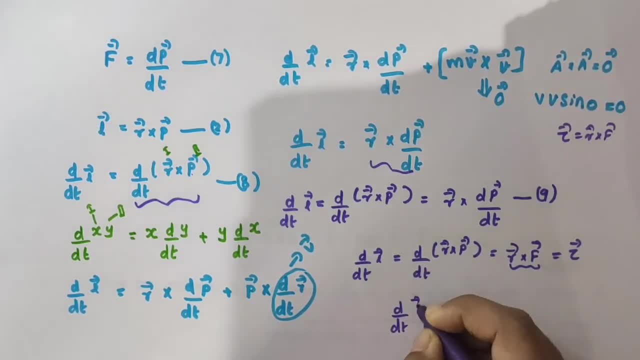 Okay, So we got d by dt of vector L is equal to what Torque. Alright, I am taking this as equation number 10.. That is, we got the relation between the moment of a force that is torque. 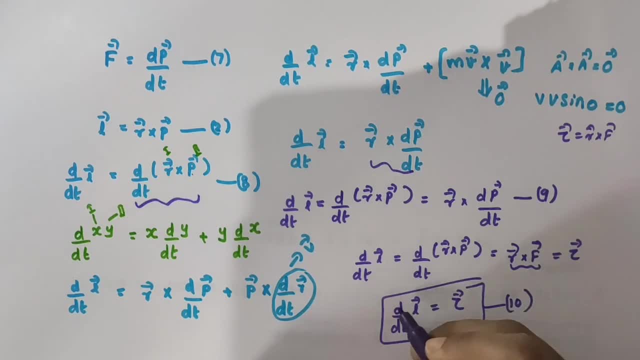 and the angular momentum vector L as d by dt of vector L is equal to vector tau. Okay, That is. the time rate of change of angular momentum of a particle is equal to the torque acting on it And this is the rotational analog of the equation: vector F equal to d. vector P divided by dt.